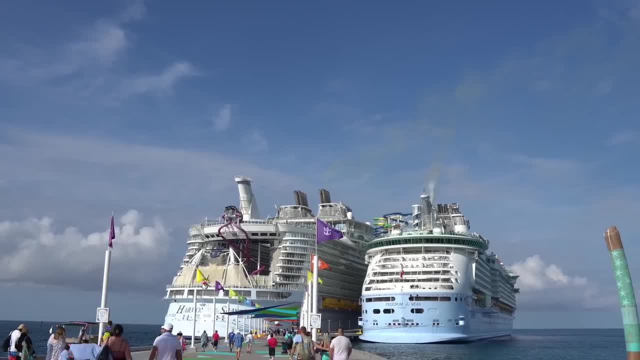 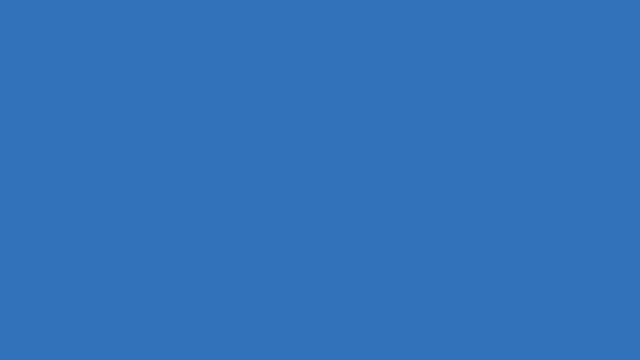 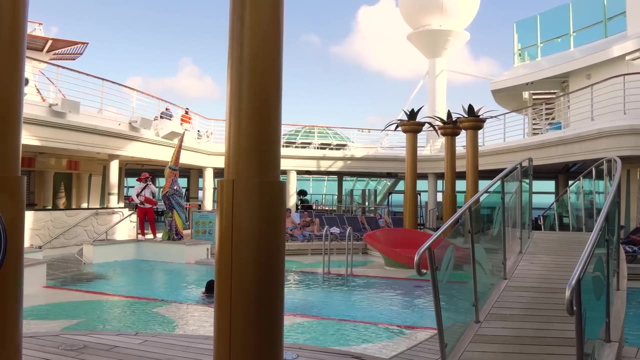 Before booking a Royal Caribbean cruise, you'll want to understand what is and is not included in your cruise, And I've got 11 fees you should know about before you book a cruise up next. Hey everyone, it's Matt from Royal Caribbean blogcom, and Royal Caribbean cruises are not. 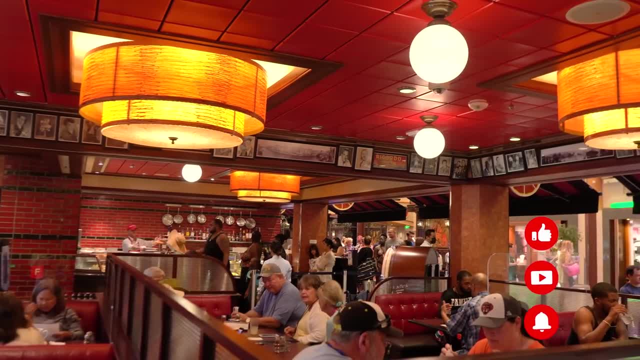 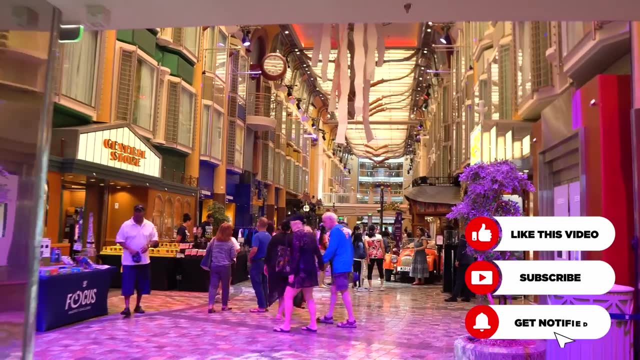 all inclusive. I don't know if that's a surprise or not, but they aren't, And there are some things that are included and some things that cost extra with it. But I think some things like short excursions are expected to cost extra, while other aspects of the cruise vacation. 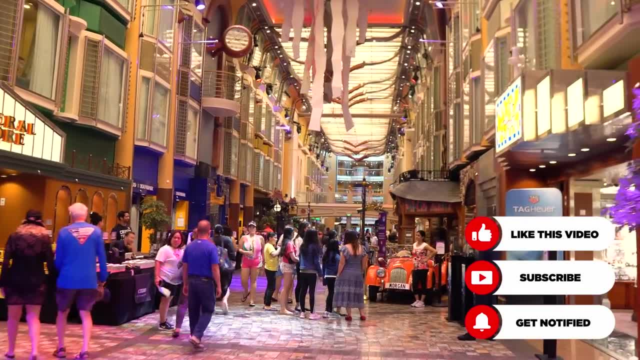 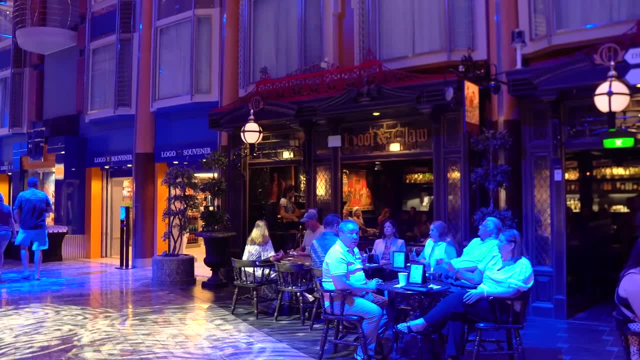 may be surprised as to the fact they're not included in your cruise fare. So I wanted to share 11 fees you should know about before booking your Royal Caribbean cruise so you can plan appropriately for your budget, Starting off with number one port fees When Royal Caribbean sends. 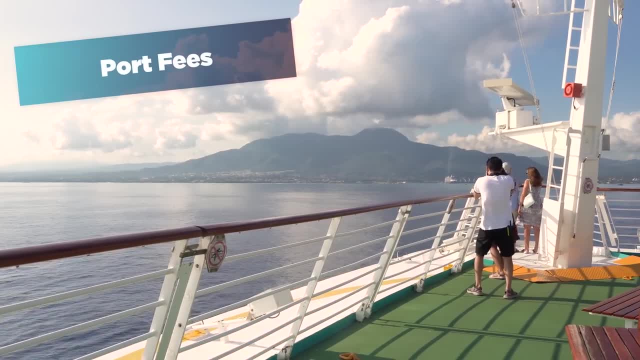 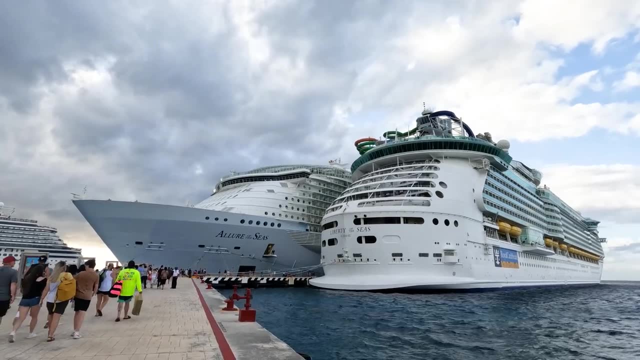 out emails advertising cruise deals. the rate does not include port fees. These mandatory fees vary based on where you're sailing to, with port fees in Alaska costing more than those in Europe or the Caribbean In July of 2025,, for instance, the port fees on a seven-night sailing to Alaska on Quantum of the. Seas cost as much as $295 per person, while the fees for a seven-night cruise to the Caribbean on the brand new Icon of the Seas cost about $185 per person. Port fees are charged by the ports of calls to the cruise lines that ships don't get to dock there for free And those fees are then. 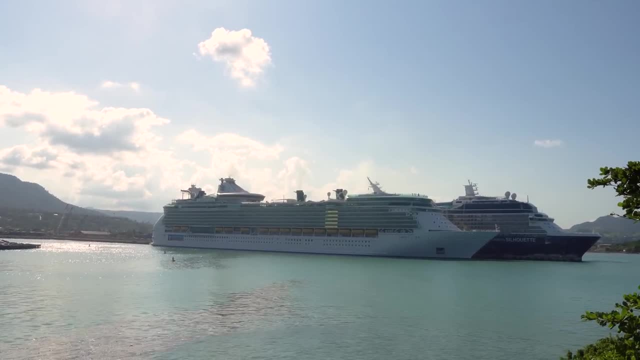 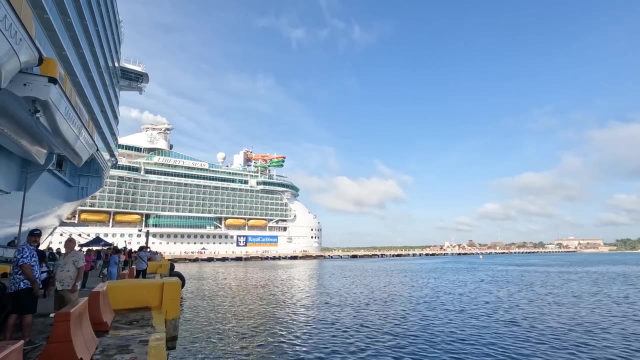 passed on to the passengers. They're usually a summation of a few different fees, including the docking fee per passenger fee, aka the head tax and the shipping fee. And then there's the pilot fee. Unlike gratuities that can be adjusted against services, port fees are paid in full by the time of final payment, and they're non-negotiable. Next up is Wi-Fi. If you want to stay connected on your cruise ship, well, you're going to need to purchase a Wi-Fi package. Unlike other cruise lines, Royal Caribbean only offers a single package for their internet access, known as the. 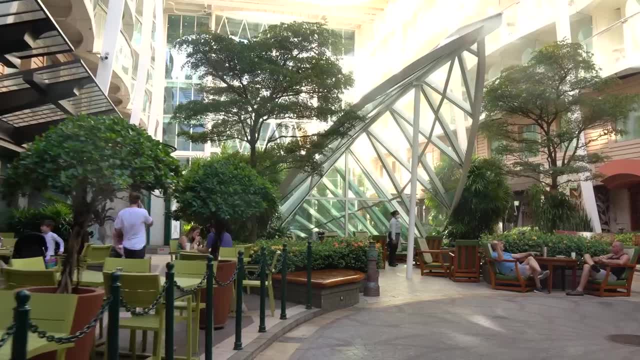 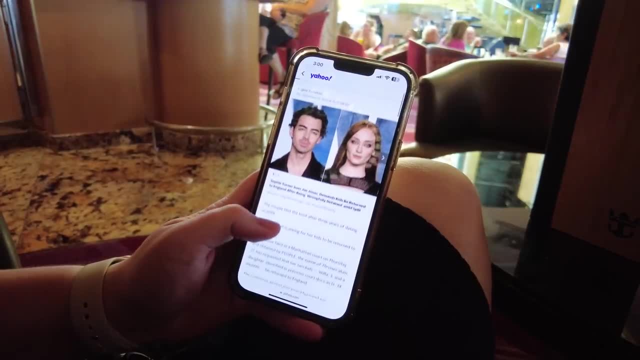 VOOM, Surf and Stream. With this package, you get 24-hour access to the internet, and there aren't any restrictions on what you can access either, and no limits per megabyte or anything like that. You can browse the web, send and receive emails, chat on Messenger apps, as well as stream your 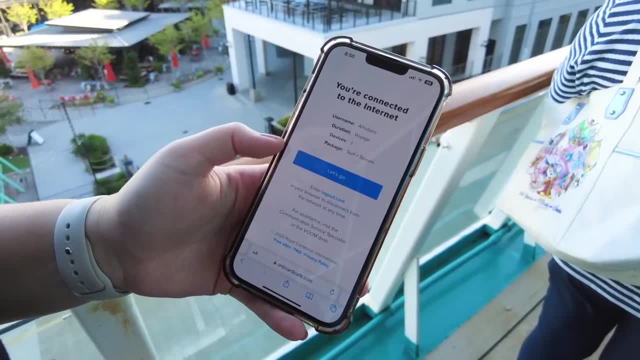 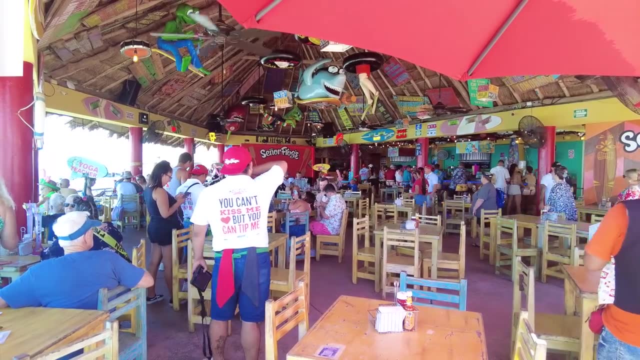 favorite TV shows, music and movies. Of course, there are ways you can check in on everyone at home without paying $20 a day, such as connecting while in port at local restaurants or coffee shops. For most, however, it's not feasible to be completely out of touch with the world. so you might want to factor in the Wi-Fi cost for your cruise Pro tip. book it before your cruise will be cheaper than if you wait to book it on board. Another extra cost you should know, As of November 2023, the automatic gratuity rate for Royal Caribbean is $18 per person per day. for a standard cabin, which means junior suites or below, and $20.50 per person per day for suites. That means that a family of four in a standard balcony cabin on a seven-night cruise can expect to pay an extra $504 for the week. You can choose to prepay gratuities before your sailing. either at the time of booking or by calling Royal Caribbean to your travel agent or have them add in your onboard account to be settled at the end of your cruise. Each guest, regardless of age, will be assessed a daily gratuity, which is then split amongst the. 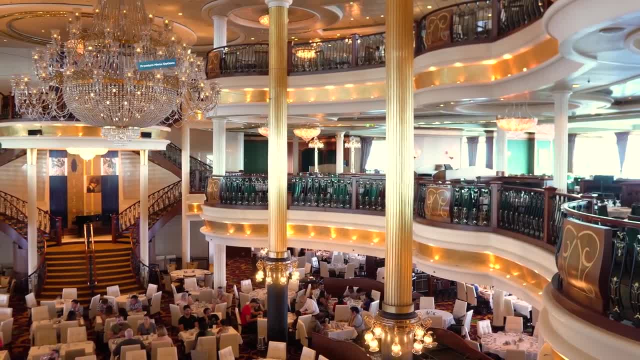 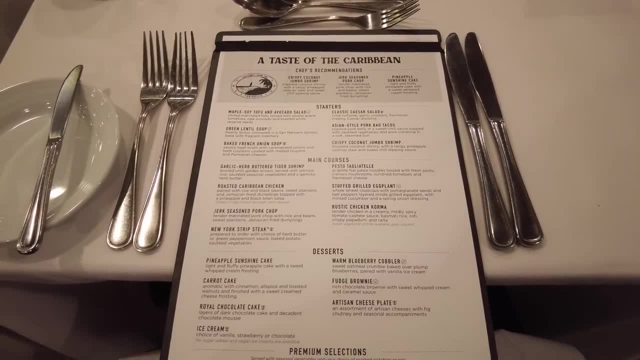 hard-working crew members. Another fee you may not be aware of are the premium menu options. So you already probably know that the main dining room is included in your cruise fare, but if you choose to eat in the main dining room, you will find some extra cost items on those menu. This. 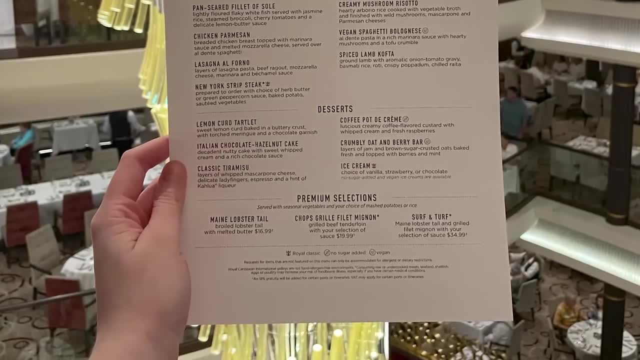 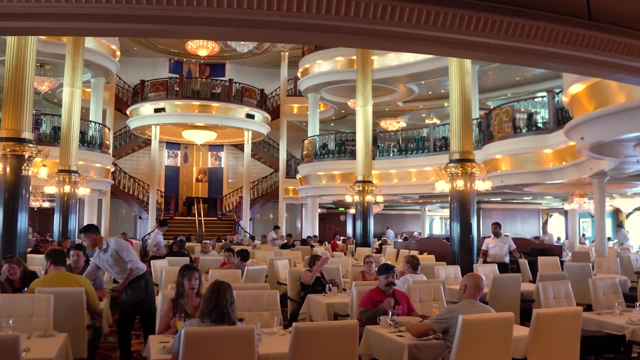 includes the main lobster tail, which is $16.99 for a single lobster, the chops grill filet mignon at $19.99, and the surf and surf, which gives you both lobster tail and filet mignon for $34.99.. Now, there'll be plenty of other things to choose from if you. don't want to pay for these upgraded offerings. If, however, you want a more intimate dining experience, well, you might go for a specialty dining meal, And, of course, specialty restaurants all cost extra, and they do range in prices depending on if it's a cover charge or an. 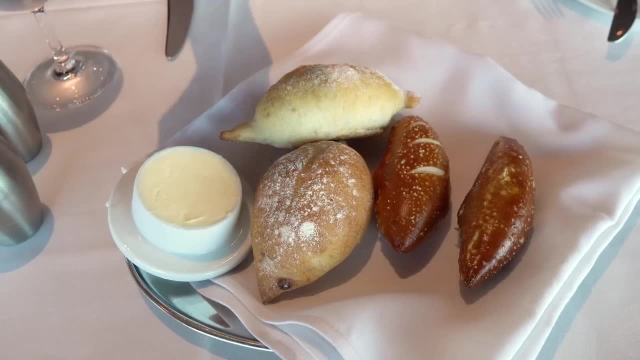 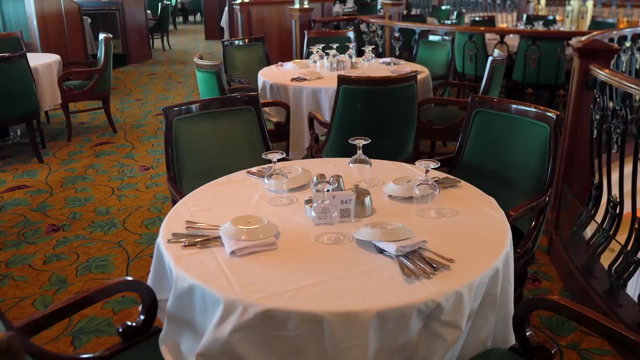 inclusive, But dining is an area you're going to want to double check on before your cruise begins because, while you can certainly have a great cruise eating purely at the Windjammer and the main dining room and just eating over there, I think inevitably a lot of people are going to want to. 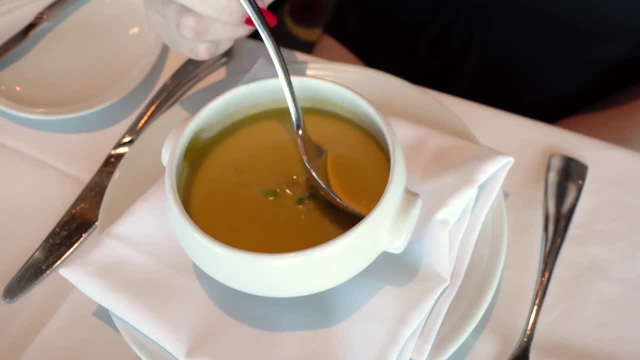 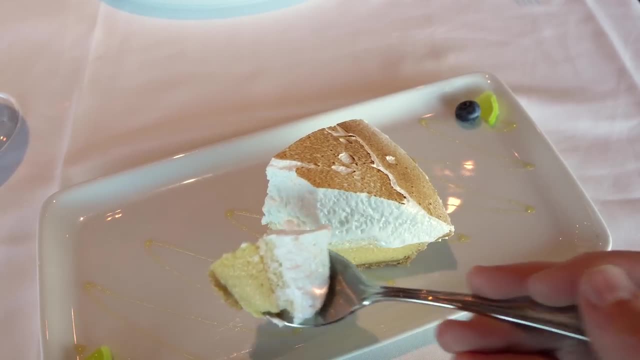 splurge a little bit and either have a dinner out at a specialty restaurant, maybe buy a dining package to eat there all the time, or, as I mentioned earlier, simply upgrade their main dining room. experience one of the nights and get filet or lobster tail while there. Whatever you choose to do, 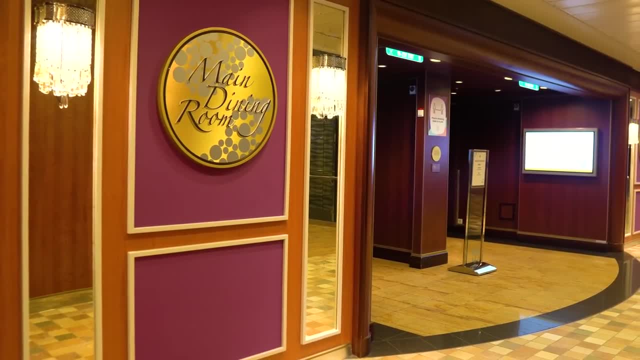 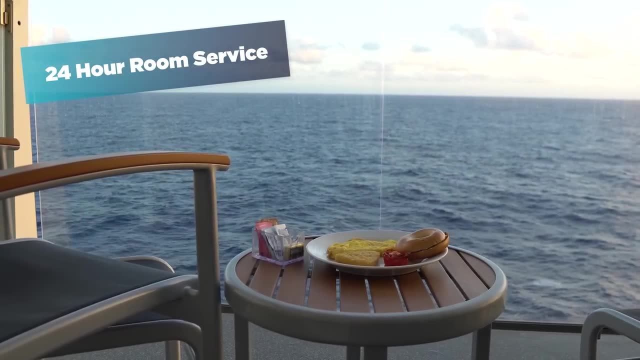 it's a really good idea to look at what those costs are and budget appropriately before your cruise. Speaking of dining, Royal Caribbean Ships offer 24-hour room service where you can have breakfast, lunch, dinner and snacks delivered right to your cabin. Whenever I cruise on a balcony, I really 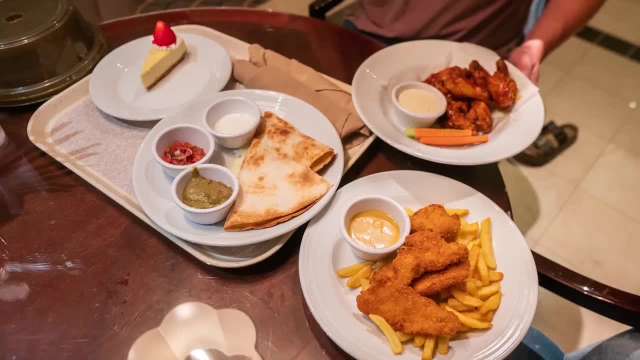 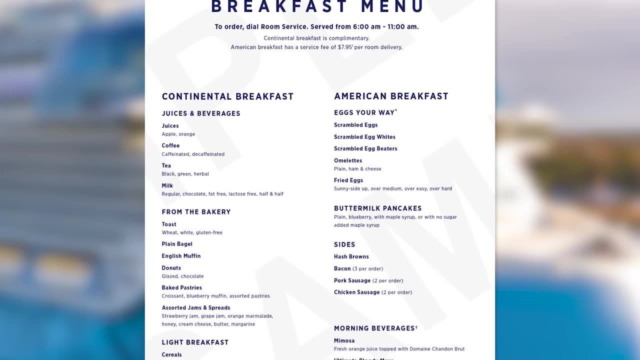 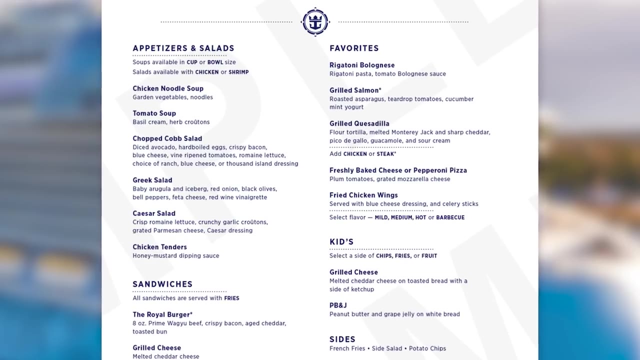 look for the opportunity to enjoy breakfast on my private balcony at least once Now. aside from the continental breakfast, all Royal Caribbean room service orders incur a $7.95 fee as well as an 18% gratuity, bringing the total cost around $9.40.. The fee is a fixed cost, meaning that you'll pay. 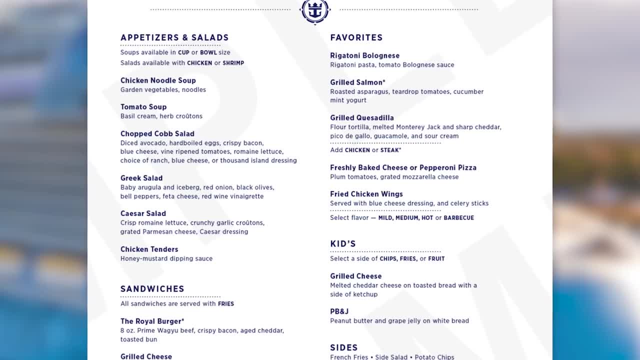 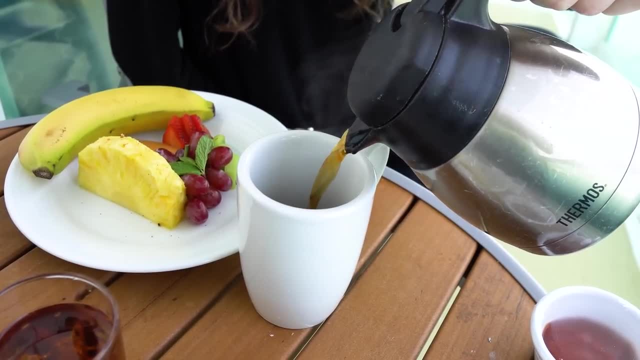 the same amount whether you order one dish or eight of them. Royal Caribbean's continental breakfast includes items like toasts, plain bagels, English muffins, assorted pastries, cereals, fruits and yogurts, If you want any hot items. 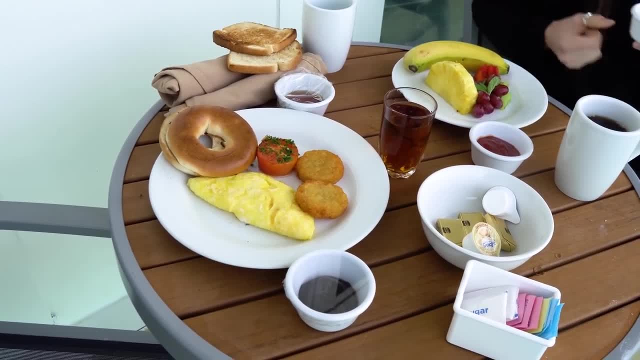 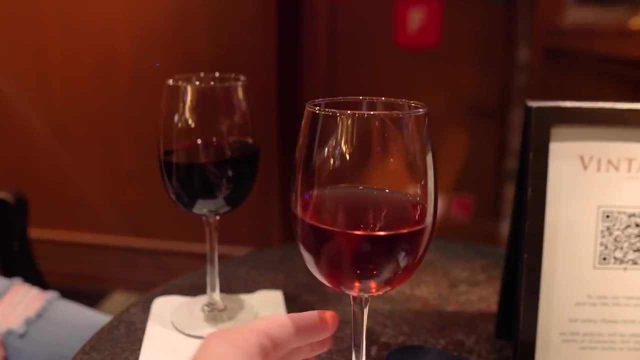 you'll have to order those and pay the service charge. Additionally, it is customary to give a small cash tip to the crew member delivering the food to your room. Another fee that I forget about all the time are corkage fees, because every guest is permitted to bring one 750-milliliter bottle of. 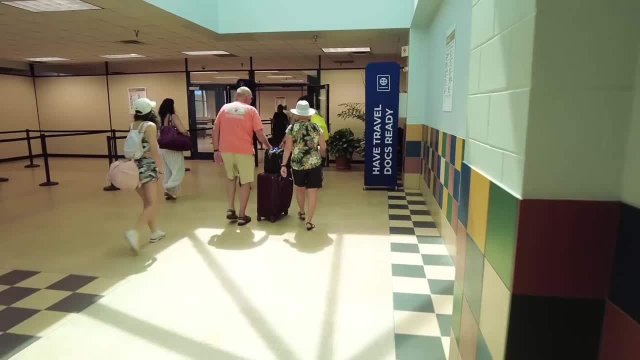 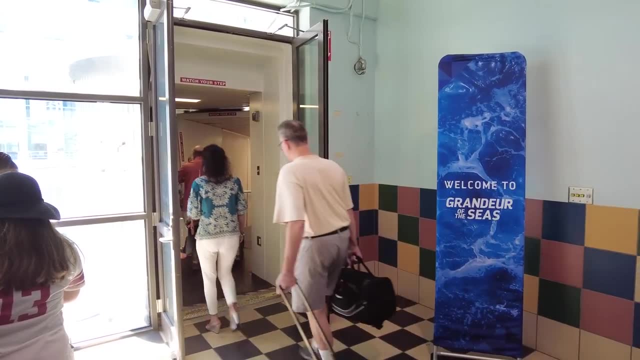 wine or champagne with them on embarkation day. While this likely won't last you the entire cruise, bringing your own alcohol on board, even in a limited quantity, is still a really good way to save money, but you should be aware that if you consume it in a platter, 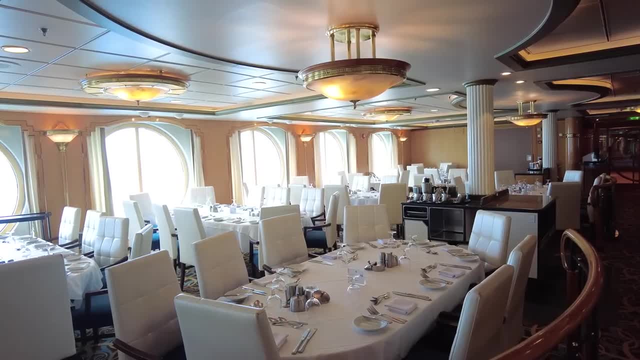 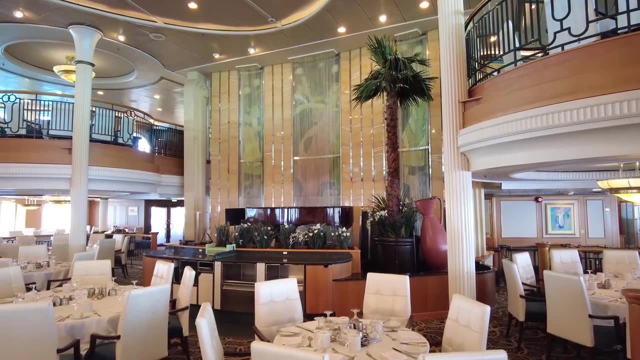 you'll be charged a corkage fee of $15 per bottle. Now I gotta admit, in my experience I'm rarely ever charged this, but it is technically a rule that you should be aware of. Then there's the thermal suite. There's no denying that the cruise ship spas are really expensive. 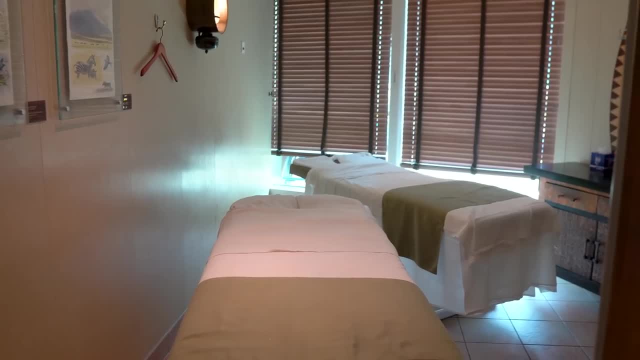 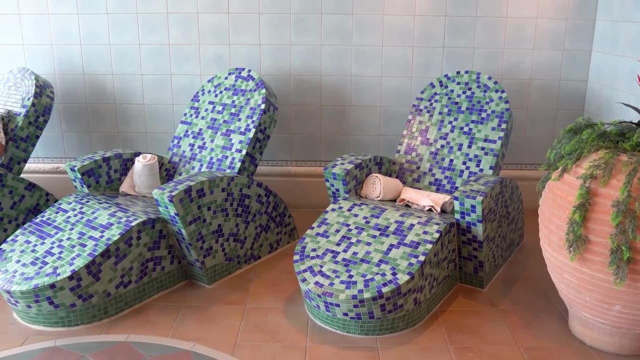 because, like, a 15-minute suite massage is going to cost like $150 or more. On Radiance, Quantum and Oasis-class cruise ships, there is a thermal suite option in which you can purchase a pass to get you access to there for the entire room. For instance, on an upcoming Quantum of the Seas cruise, the list price for a seven-day pass is $125,, which is cheaper than a 15-minute treatment that you'll only be able to enjoy once, as opposed to being able to enjoy the thermal spa. 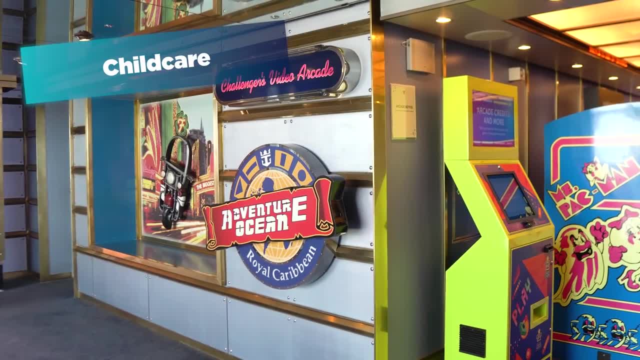 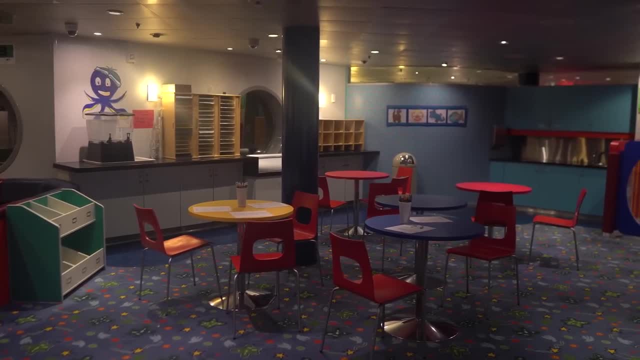 for the entire length of the cruise. Then there's child care, Don't worry. Adventure Ocean programming is complimentary for kids between the ages of 3 and 12 during the day. An hourly rate does apply for 10 pm, though That's a separate program. 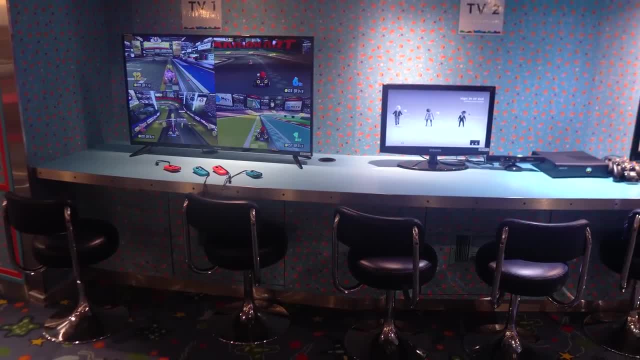 altogether. but the good news is, if you've got kids or teens, that's included in the program. You don't have to worry about that. If you have kids or teens, that's included in the program. You don't have to worry about that If you have kids or teens. 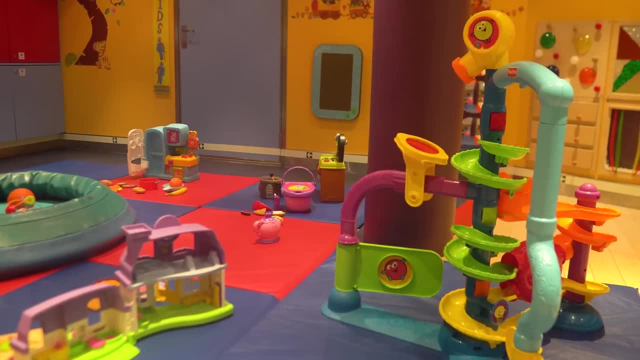 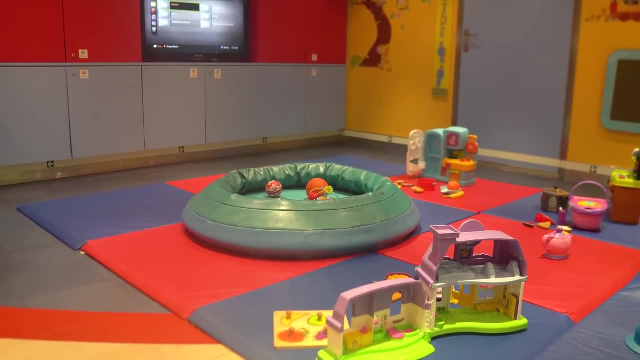 that's included with your cruise fare, But kids under the age of 3 cannot partake in the complimentary programming. If you have a child that's between 6 and 36 months old, then you'll need to go to the Royal Babies and Tots, and that's a great option. It's a nursery drop-off. 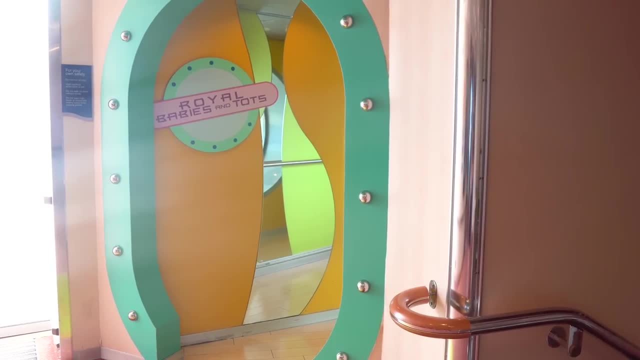 for guests between the ages of 6 and 36 months, as I mentioned, and the cost is $6 per hour between 9 am and 6 pm, and then $8 per hour from 6 pm until midnight. 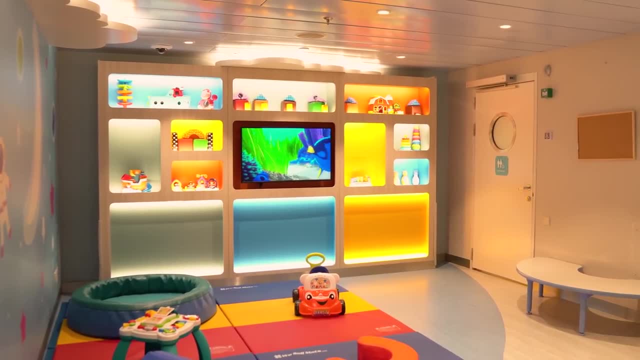 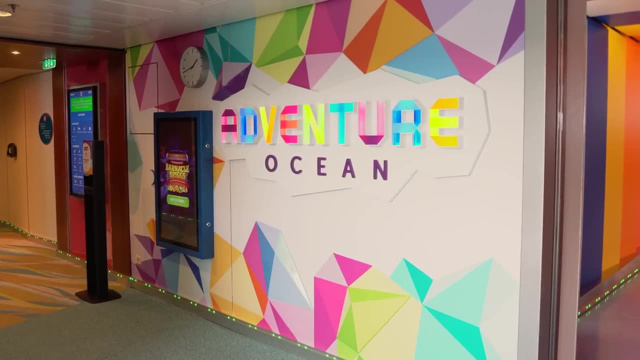 Regardless of where your child has to go, there will be age-appropriate activities for them to enjoy, while parents get some much-needed alone time. I think it's the best money you'll ever spend on a cruise ship, but be aware that child care may cost you extra. 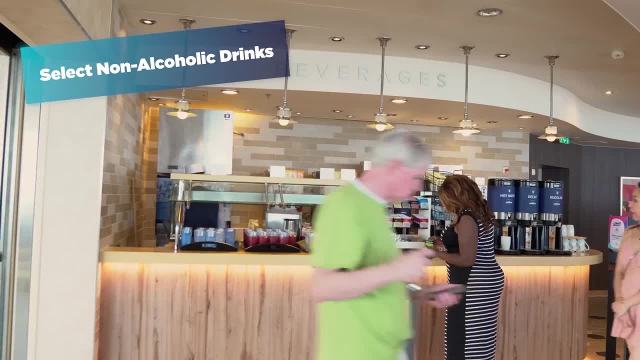 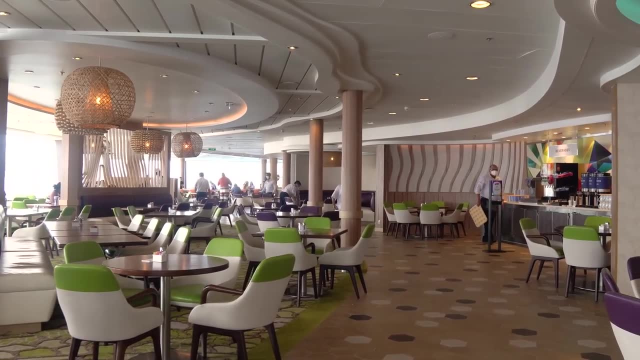 And then, of course, there is select non-alcoholic beverages. Your base fare includes things like water and milk and tea, coffee, lemonade, iced tea, flavored waters, juices at breakfast and hot chocolate, But if you want something else, like specialty coffees or sodas, or mocktails. you either need to pay for each drink individually or go for a Royal Caribbean drink package. As of December 2023, most zero-proof cocktails are $7, with specialty coffees at Cafe Promenade and Cafe Latitudes between about $4 and $5.50. Soda on board Royal Caribbean cruise ships are $3.50 each. So Royal Caribbean offers two different non-alcoholic packages, though that might be able to save you money: The Classic Soda Package and the Royal Refreshing Package. The Refreshing Package is more expensive, obviously, but it includes all non-alcoholic. 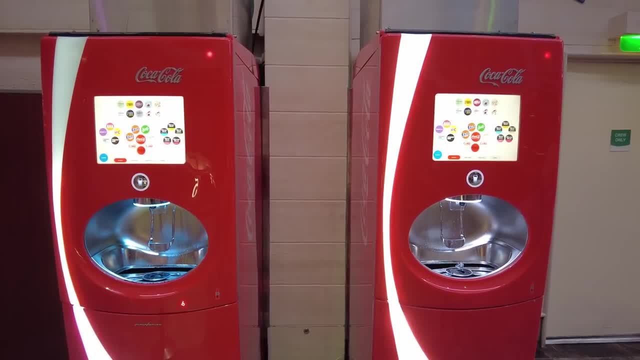 cocktails, mocktails, Coca-Cola freestyle beverages and soda refills at any venue, bottled still in sparkling water and soda refills. So if you're looking for a drink, you're going to want to go with the Royal Caribbean. The Royal Caribbean offers two different non-alcoholic packages, though that might be able to save you money: The Classic Soda Package and the Royal Refreshing Package. The Royal Caribbean offers two different non-alcoholic packages, though that might be able to save you money, Still in sparkling water, specialty teas and coffees. 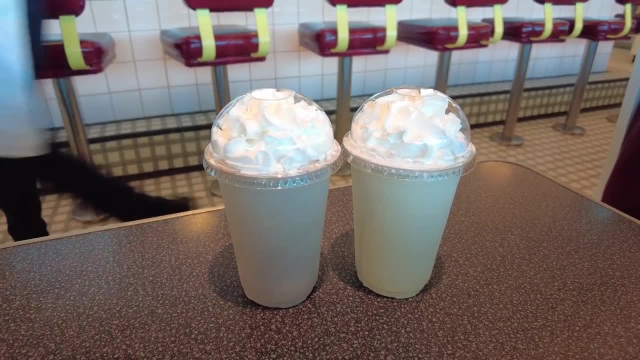 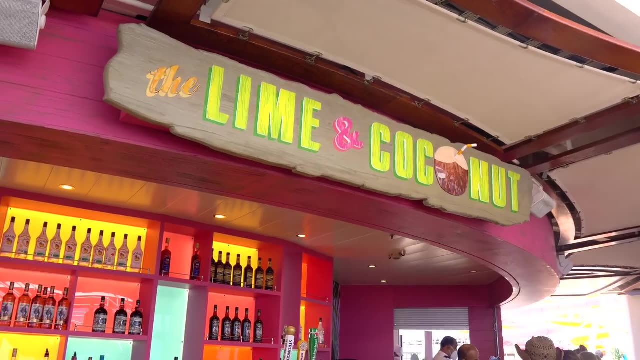 shiny rocket shakes and freshly squeezed juices. The Classic Soda Package includes just soda, though, so you'll have to pay extra for anything that's not a soda drink. And then, of course, there's alcohol. Maybe this is a surprise to you, maybe it's not. 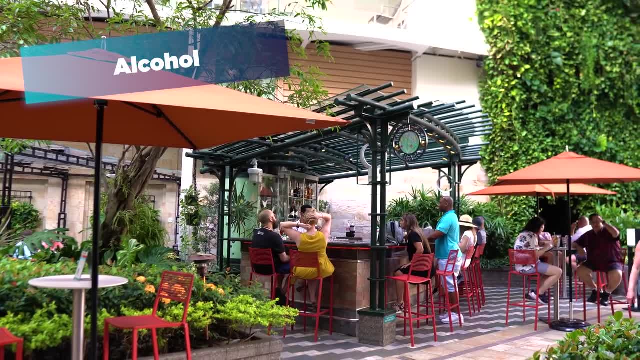 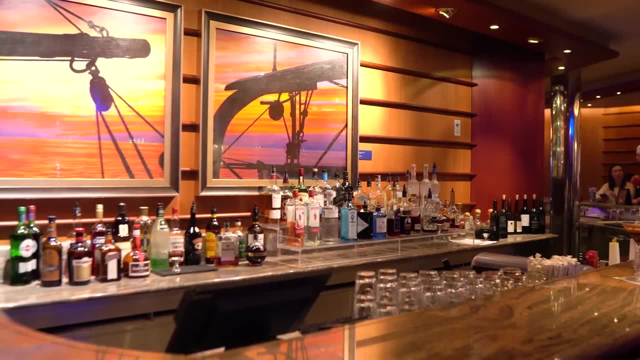 but alcohol beverages cost extra on a Royal Caribbean cruise. You can either pay for them individually or you can get a drink package. A cocktail will probably cost you between $10 and $15.. A beer is like $8 or so And, of course, the cost of a beverage package will probably be between $10 and $15. A beer is like $8 or so. 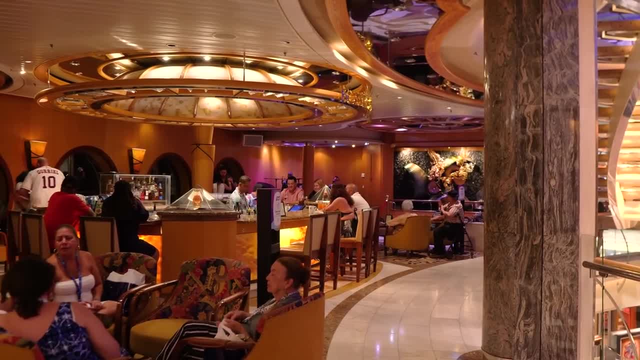 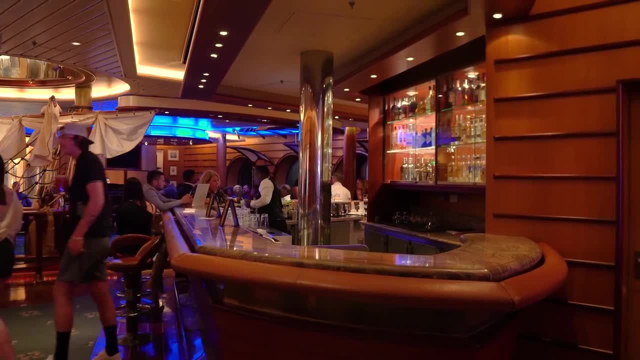 And, of course, the cost of a beverage package like the Deluxe Beverage Package, which is the only alcoholic package offered, is going to range depending on your sailing. Usually it's between like $60 and $105 per person per day. 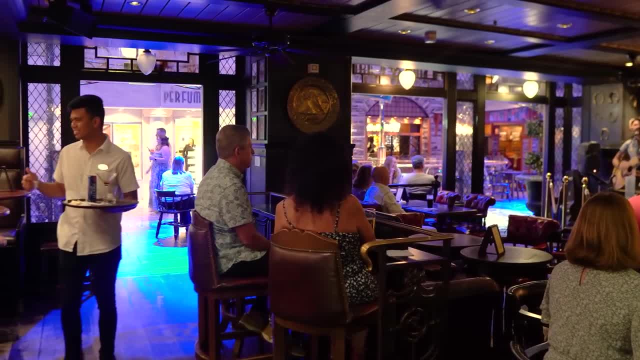 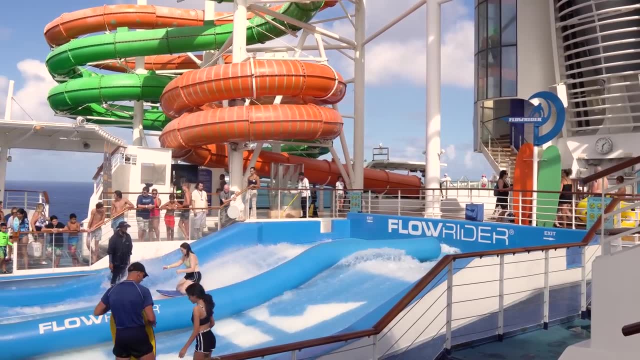 No matter which drink package you choose, you will absolutely save money by pre-purchasing the drink package before your cruise. Don't wait to book it on board the cruise ship. And lastly, there are certain onboard activities that will cost you extra you might not be aware of. Royal Caribbean is known for packing your ships full of onboard. 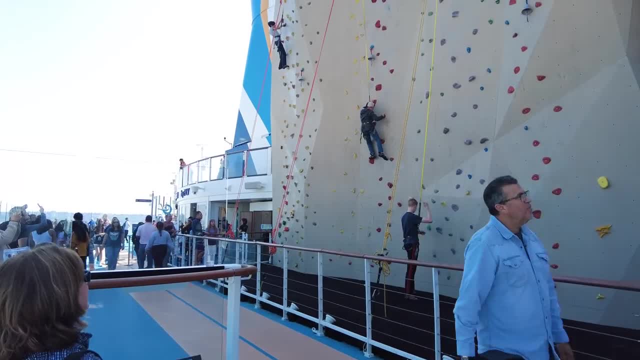 thrillers. So if you're looking for a drink package that will be a good fit for your cruise, you'll have to pay extra, Depending on which class you sail on. you'll find anything from ice skating rinks, skydiving simulators, bumper cars, zip lines, water slides and more. 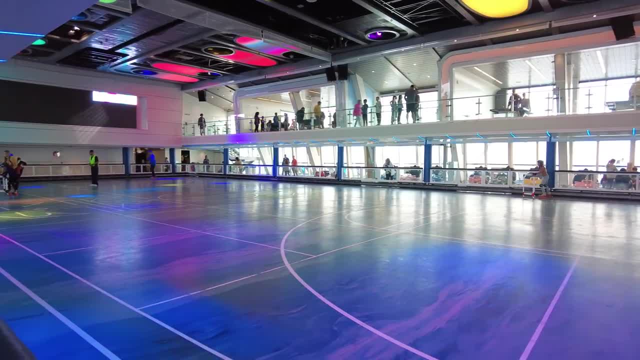 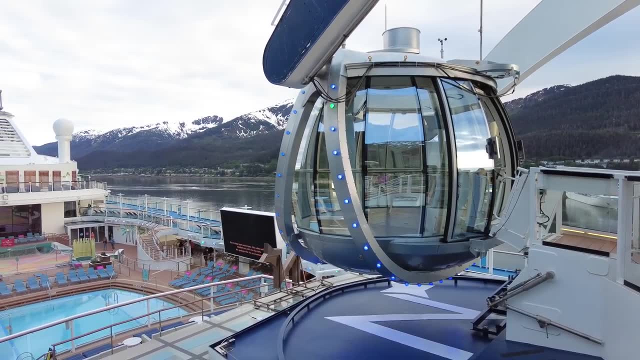 The majority of activities are included in the cost of your cruise, but there are some that cost extra, such as the North Star Observational Pod on sea days costing extra, and fitness classes. In addition, if you want a Floor Rider lesson, whether it's private or a group- 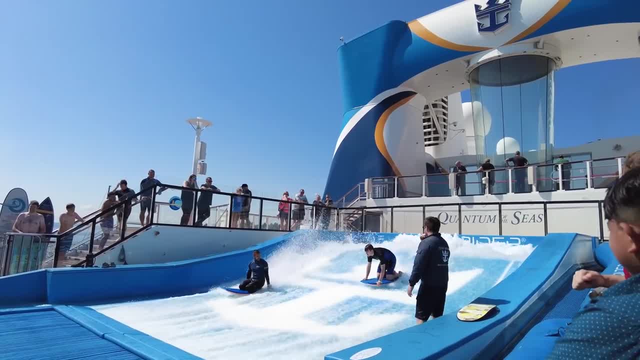 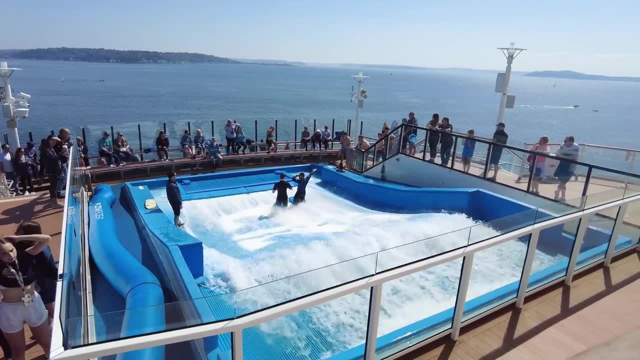 you'll have to pay extra for that, with the latter being the cheaper option. Usually, the group lessons cost around $60 per person. So there you have it: A look at the 11 most important cruise fees. you should know they're going to cost extra. 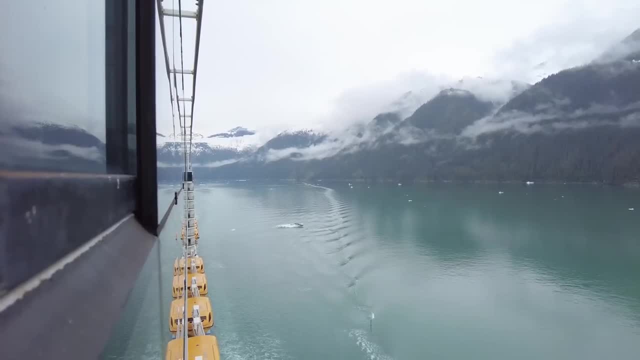 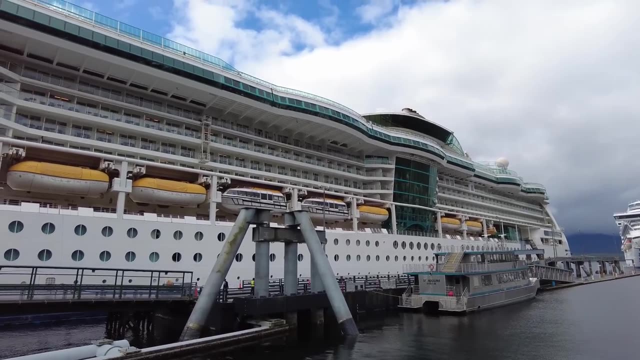 and how to maybe mitigate them a little bit. bring those prices down. Let me know in the comments below which of these are a surprise to you and which of these are a must-do. I mean poor fees everyone's going to pay for, But which of these do you go for?